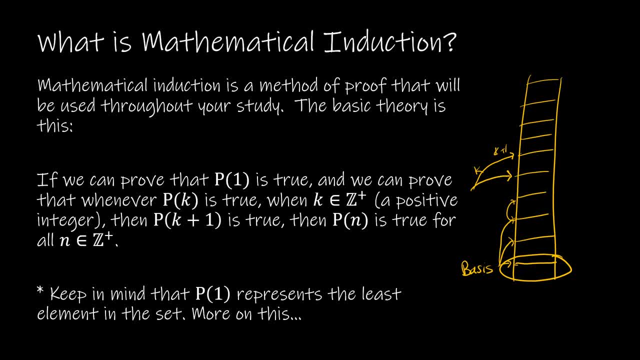 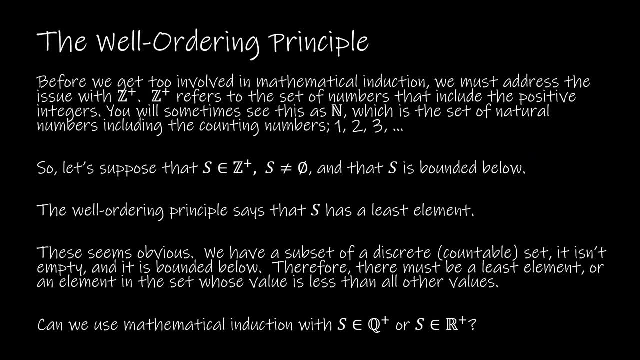 with a different value. that is the least element And that brings us to the well-ordering principle. So before we get too involved in our mathematical induction study, we have to talk about z plus. Z plus means the positive integers, So that starts at the number 1, so 1,, 2,, 3, and so on. 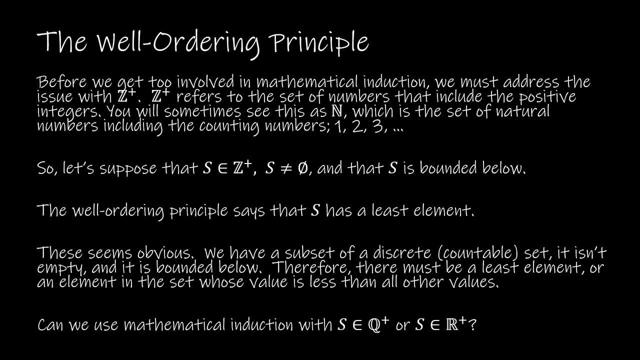 You might also see that referred to as the natural numbers. So the whole numbers include 0, and we don't want to include 0. So the natural numbers are just the counting numbers: 1,, 2,, 3,, 4, and so on. So what we're going to say is our set S is an element of z plus, So all of the 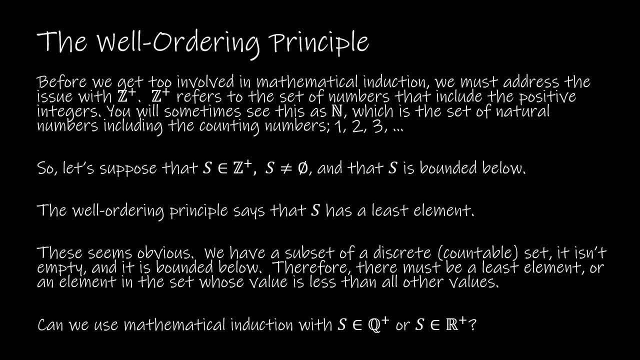 elements are positive integers. S is not equal to the empty set, so S is not empty And that S is bounded below. So bounded below is our basis step. So this is very important, that our set is bounded below because we need a first element. So the well-ordering principle. 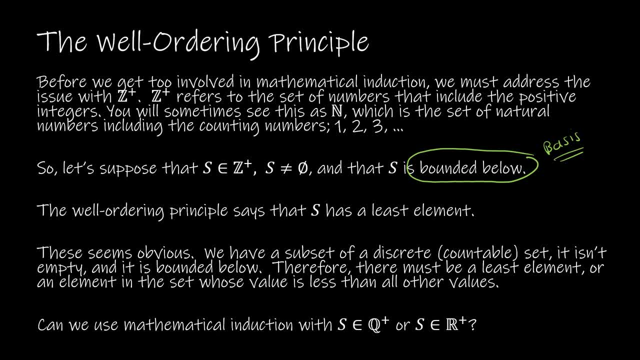 says that S has a least element, and that's what we need in order for mathematical induction to work. So obviously it seems obvious. We have a subset of discrete which just means countable objects. It's not a set of discrete which just means countable objects. So we have a subset of. discrete, which just means countable objects, And that's what we need in order for mathematical induction to work. So let's say we have a subset of discrete, which just means countable objects, And that's what we need in order for mathematical induction to work. So we have a 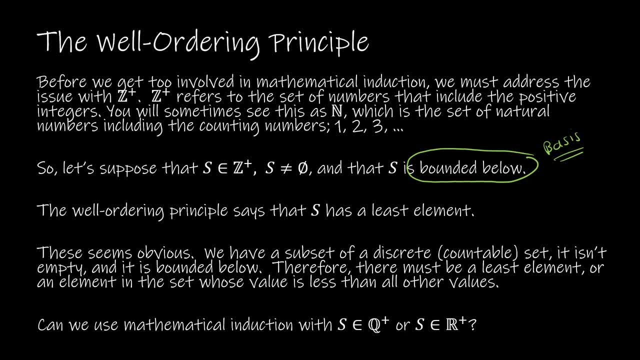 bounded set of Z plus. So our set S is not empty, It's bounded below. Therefore, there must be a least element or an element in the set whose value is less than all the others. Now it's important that we're using Z plus here, because if you think about Q plus, remember Q is the 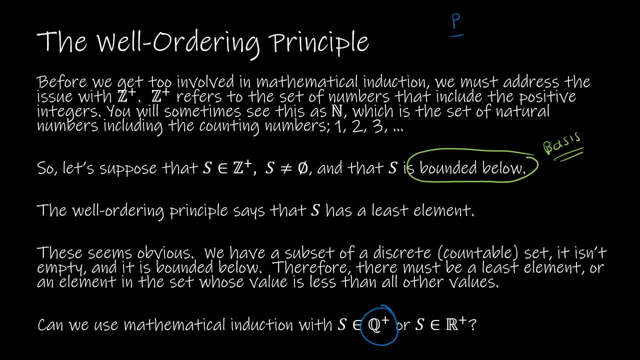 rational number. So that's anything that we can write as P over Q. Is there a least element in that? Well, we could say one half. Well, we know that a number less than that is one half. So we than one-half is one-third. A number less than one-third is one-fiftieth. A number less than 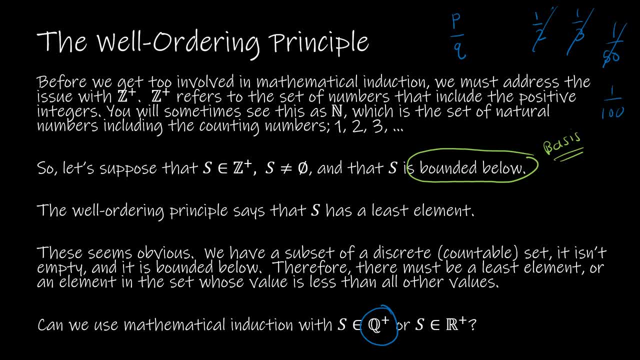 that closer to zero is one-one-hundredth, And you can see that we could never get to a least element because we can always make the denominator larger. Same thing would go for all real numbers. So it's very important that we're using the integers here for mathematical induction. 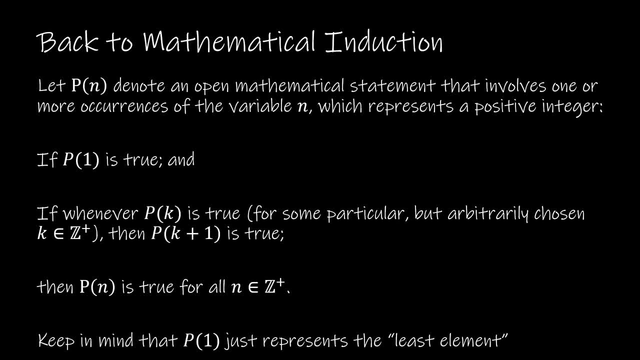 So let's get back to mathematical induction. We're going to let p of n denote some mathematical statement. So, as we are working through mathematical induction, we are going to be very specific about what p of n represents. So it's going to be some statement that involves: 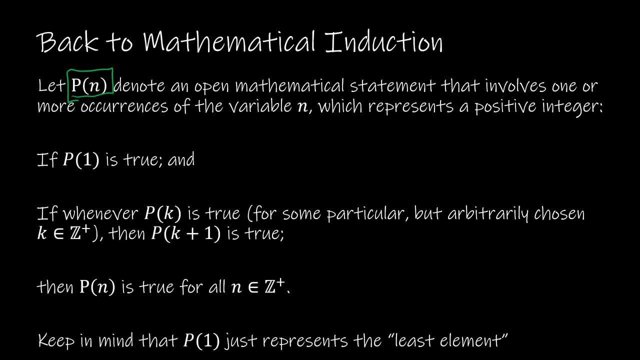 one or more occurrences of the variable n, which represents a positive integer. Remember, that's that z plus. Then we're going to prove p of 1 is true. And remember p of 1, just represents the least element, So it might be 1, it might be 2, it might be 45.. 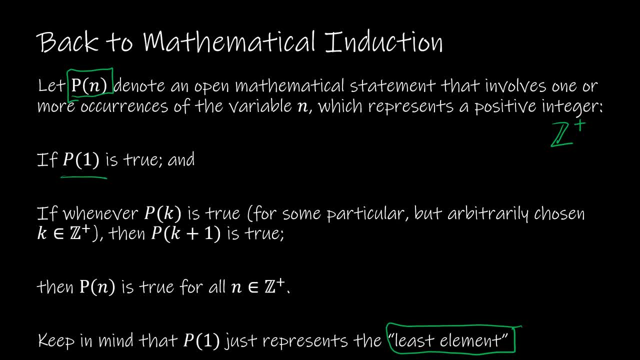 And then if, whenever p of k is true for some particular but arbitrarily chosen value- that is also, of course, a positive integer- then p, k plus 1 is true. then we know that it's true for all values. So let's take a look at an example together. We're only going to do one. 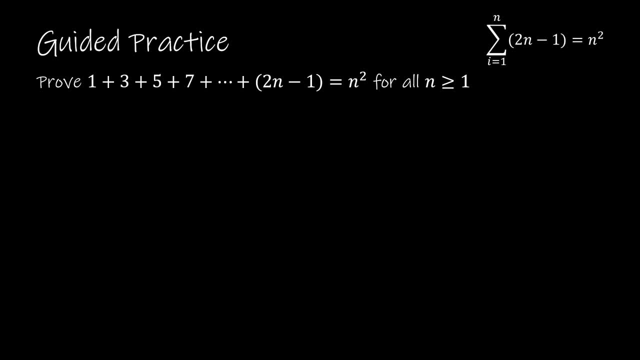 particular value. We're only going to do one particular value. So let's take a look at an example together. We're only going to do one particular value. We're only going to do one proof in this video and we're just going to work through it together And remember that we're 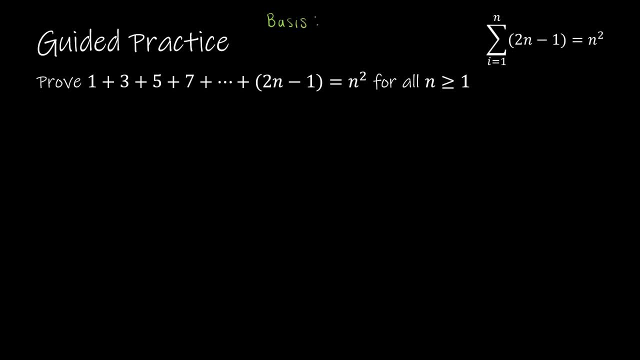 going to show, just so we remember what we're doing, where we're going. here we've got a basis step and we've got an inductive step And our basis shows that p of 1 is true And our inductive 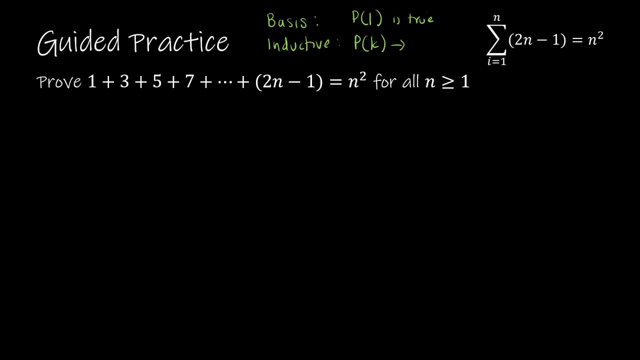 step says: if p of k is true, it implies that p of k plus 1 is true. So that's where we're going here. Now the question that we're going to solve together is to show or prove that 1 plus 3 plus 5. 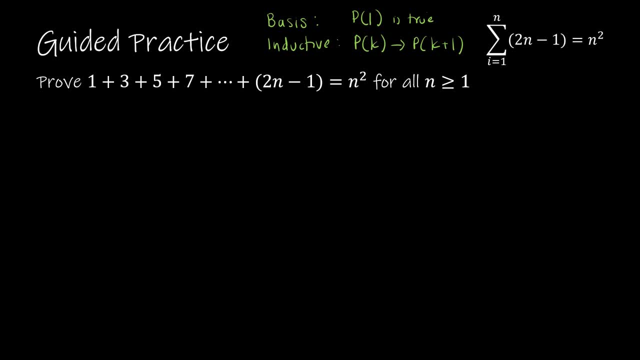 plus 7 and so on, plus 2n minus 1, which is essentially all the odd integers, that the sum is equal to n squared. So I've shown you two different ways how the question might be given to you. So this is obviously the original for all of n greater than or equal to 1.. 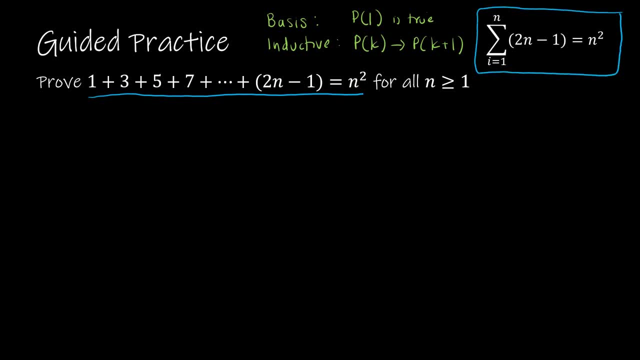 Or they might actually show you the summation, Or they might say: find the formula for the sum of the first n odd integers and then prove your conjecture. So we're going to go ahead, and we obviously didn't have to find it. 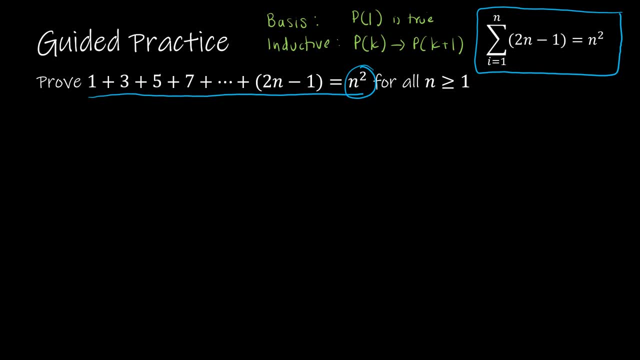 We were given that the sum is actually equal to n squared, And we will go through in the next video, one where we actually have to find the formula ourselves. So stay tuned for that. So, from here, what I'm going to do is: 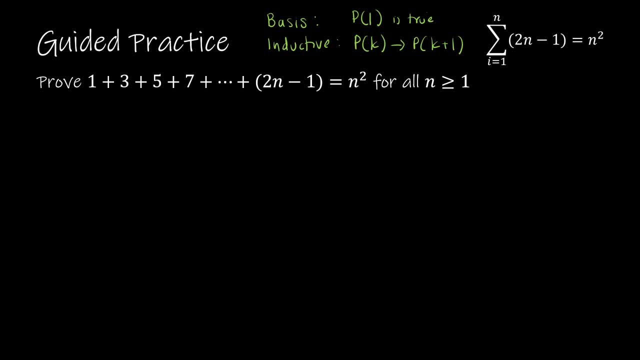 every first step which I didn't write in green up above. shame on me. My first step is always to say let p of n be the statement And then basically say what it is that I'm trying to prove. So I'm going to say 1 plus 3 plus. 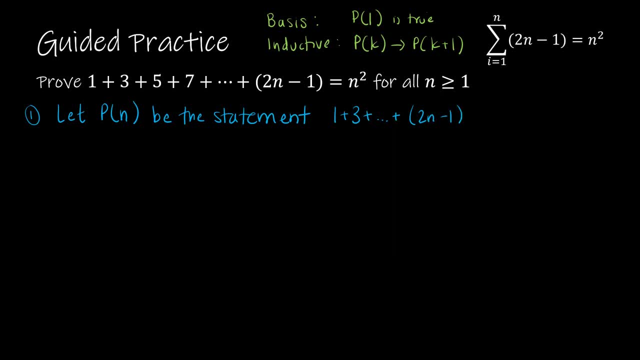 so on and so forth. plus 2n, minus 1 is equal to n squared. That is what I'm trying to prove for all n greater than or equal to 1.. That's the first step. So first step is write p of n. tell what it is that you're proving. 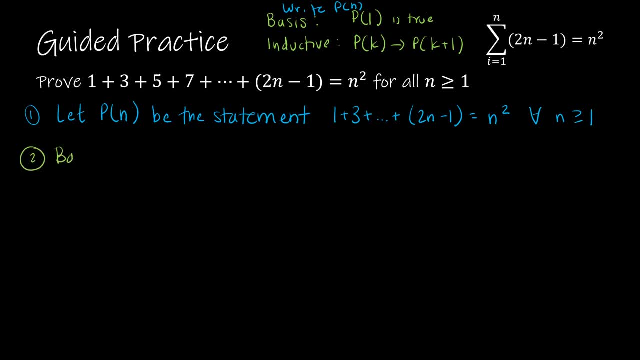 Then we're going to look at the basis step. And again, our basis step says: start at the least element in your set of values. So we're looking at values. n is greater than or equal to 1.. So 1 is our first value. 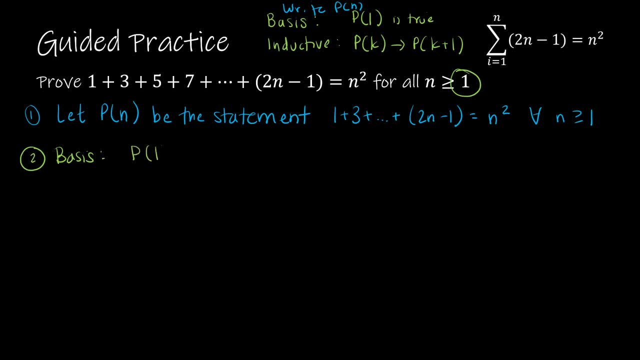 So we have to show that P of 1 is true. So P of 1 says that 1 is equal to 1 squared. Well, because n squared obviously would be 1 squared, 1 is equal to 1, and therefore that one checks out. 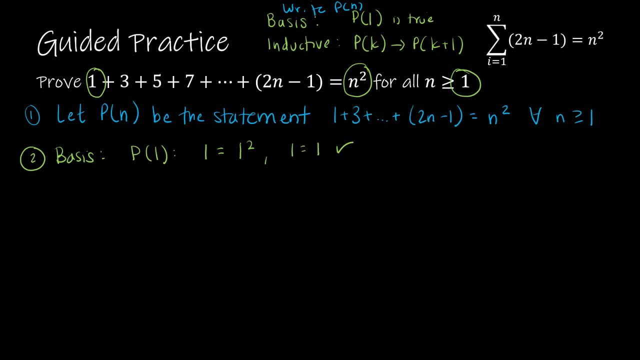 So the basis step is proven. Then we're going to look at step 3, which is the inductive step, And the inductive step has actually parts of its own. So for the inductive step, remember we're going to show that P of K implies P of K plus 1.. 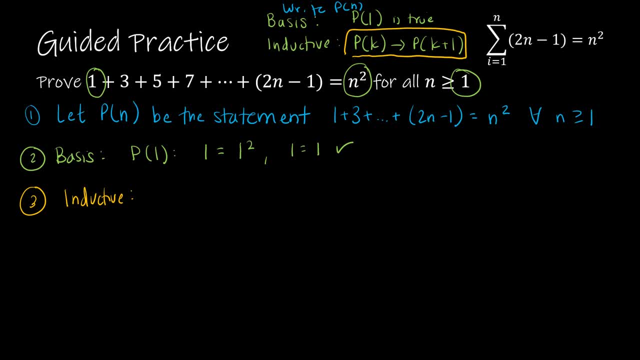 So for the inductive step we're going to give first the inductive hypothesis. So I'm just going to write IH for inductive hypothesis, The inductive hypothesis. The inductive hypothesis is that P of K is true. So my inductive hypothesis says: assume that 1 plus 3 plus 5 plus so on, plus 2K minus 1.. 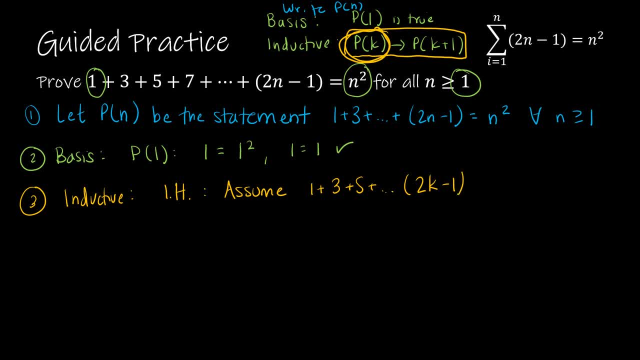 And yes, you should change the value of your variable, because we're not using it for n, We're using it for some arbitrary value of K. So we're assuming that that is equal to K squared. So if that's true, then I'm going to include the what to prove. 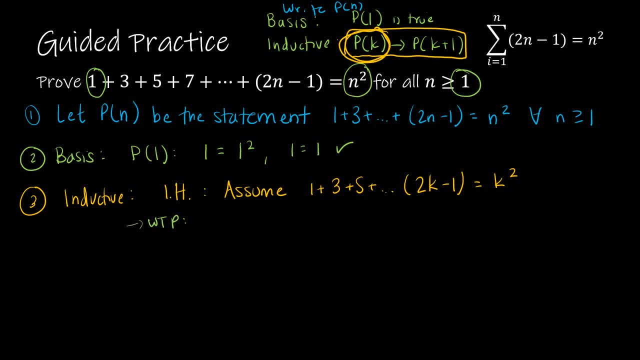 Now this is not a required step for in general, I guess, But if you're in my class you should be writing the what to prove, So I know that that's what you're trying to prove. So I'm trying to prove that: 1 plus 3 plus 5 plus so on, plus 2K minus 1.. 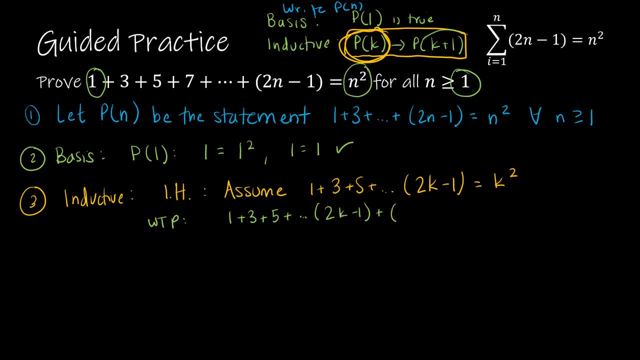 Plus the next value, which would be using K plus 1 for K. So 2 times the quantity of K plus 1 minus 1 equals K plus 1 squared. So again, that's what I'm trying to prove, And I'm going to prove it by starting with the assumption that my inductive hypothesis is true. 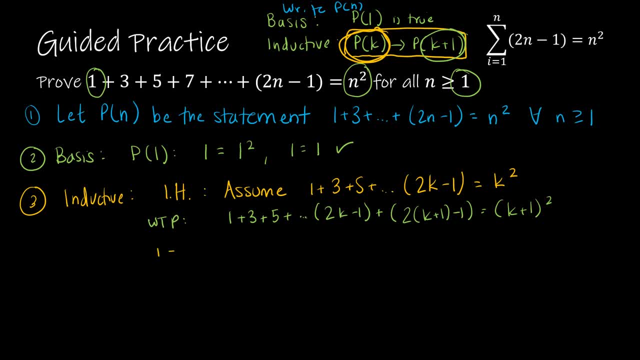 So here's my proof. I know that 1 plus 3 plus 5.. Plus so on, plus 2K minus 1 is is equal to K squared, based on my inductive hypothesis. So I'm really just rewriting my inductive hypothesis. 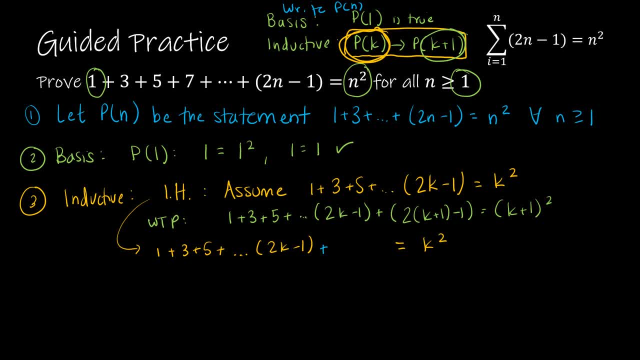 And then I'm going to add the same thing to each side. So I'm going to add 2 times the quantity of K plus 1 minus 1.. And I'm just going to clean that up before I add it. So this would be 2K. 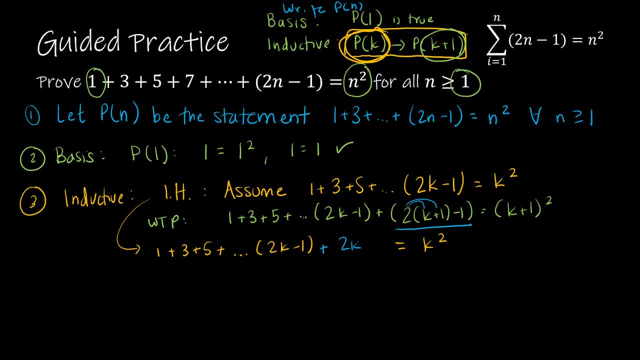 And then I have plus 2 and minus 1.. So it's really 2K plus 1.. Now it's important here that I add the exact same thing to each side. So that's what I've done. Now, on the left hand side of my equation, I have exactly what I want. 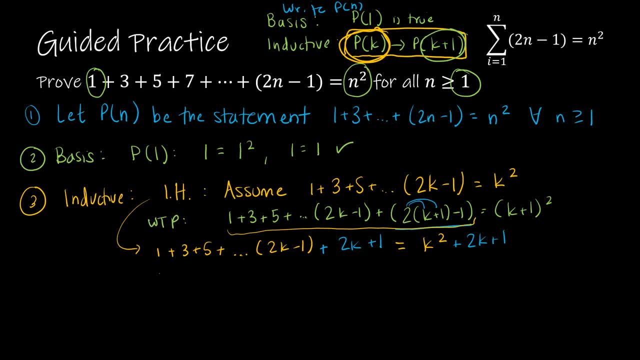 I have the statement that I'm trying to prove. So I have 1 plus 3 plus 5 plus, so on, plus 2K minus 1 plus 2K plus 1.. And on the right side, remember what am I trying to prove? 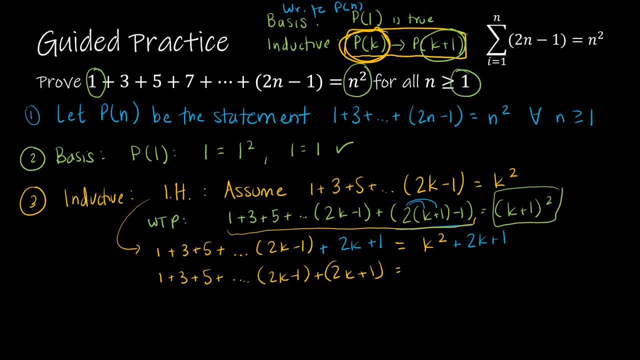 I'm trying to prove that's all equal to K plus 1 squared. So on the right side I have K squared plus 2K plus 1.. Well, good thing, I know how to factor. I'm looking for two values that have a product of 1 and a sum of 2.. 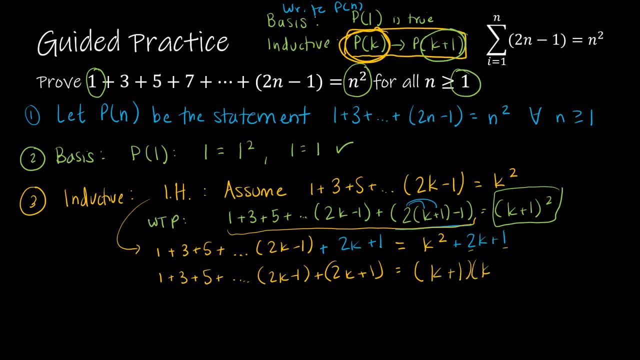 And that happens to be K plus 1, and then K plus 1, which, of course, is exactly what I want, which is K plus 1.. And then I have 2K plus 1.. And then I have 2K plus 1.. 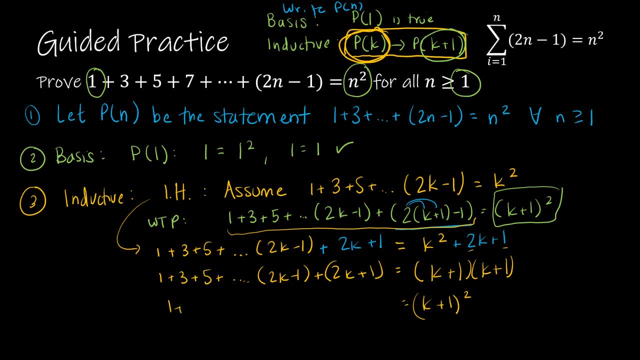 And then I have 2K plus 1 squared. So I have very simply, using mathematical induction, proven exactly what it was that I wanted to prove, which is that adding 2K plus 1 to each side does in fact result in my statement. 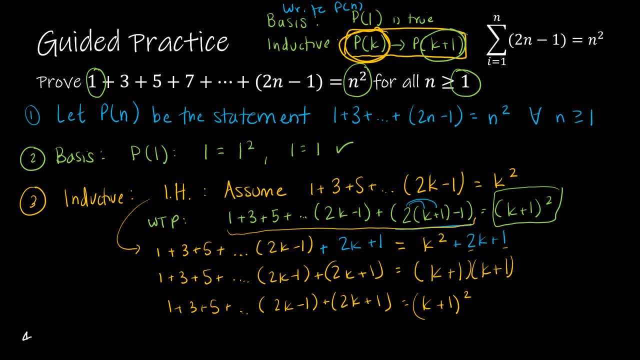 Now, the very, very last thing that I should do is say: because The basis is true, and P of K implies P of K plus 1, then P of N is true, for I'm going to use for all N greater than or equal to 1.. 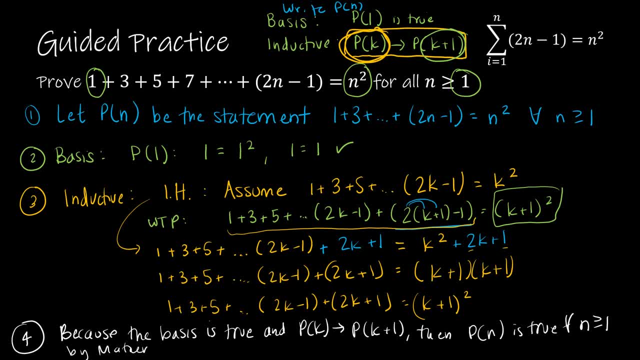 So I'm going to use for all N greater than or equal to 1.. So I'm going to use for all N greater than or equal to 1.. And then, if I do specify it, I'm going to say 1 minus 1.. 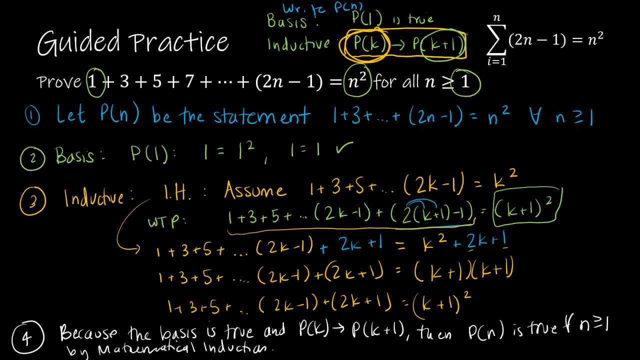 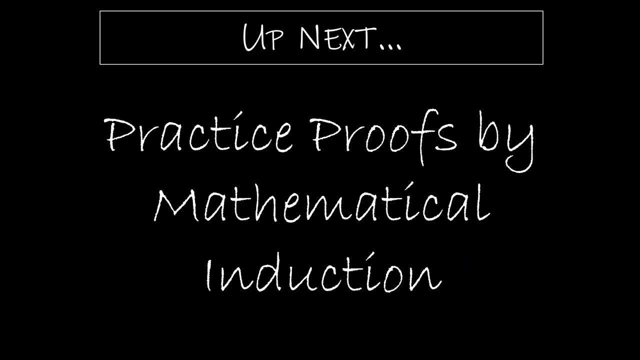 So I'm going to do a number of times by mathematical induction. So that is a great proof. you've got all of the parts that you need. In our next video, we're just going to focus on doing some practice. proofs by mathematical induction. In our next video we're just going to focus on doing some practice proofs by mathematical induction.